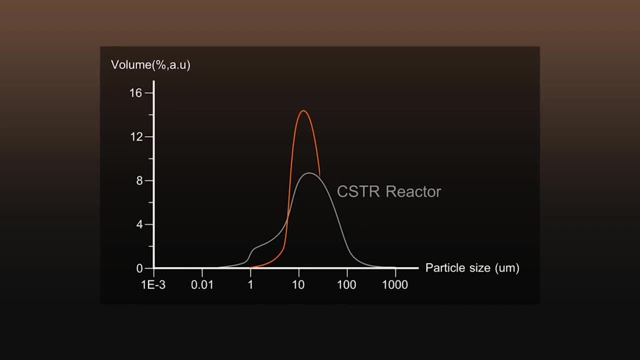 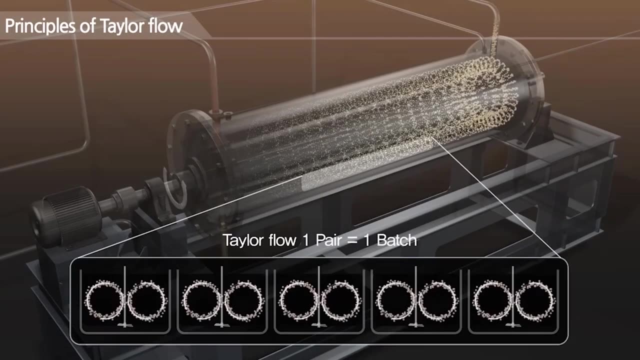 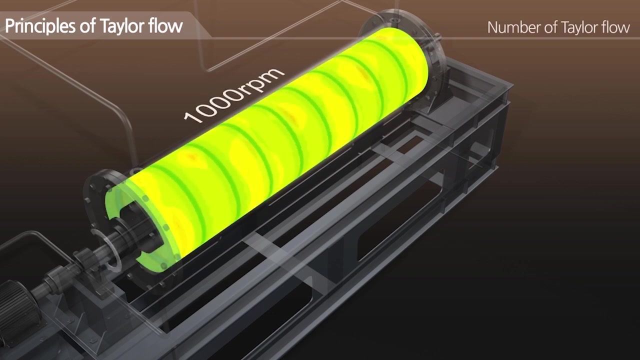 They combine the advantages of tank and tubular type reactors in the production of high purity materials under continuous flow. Their flow reactors are designed to exploit specific turbulent mixing through Taylor flow. The significance of Laminar continuous Taylor flow reactors is that they can reduce reaction times, increase purity, offer full control over reactions. 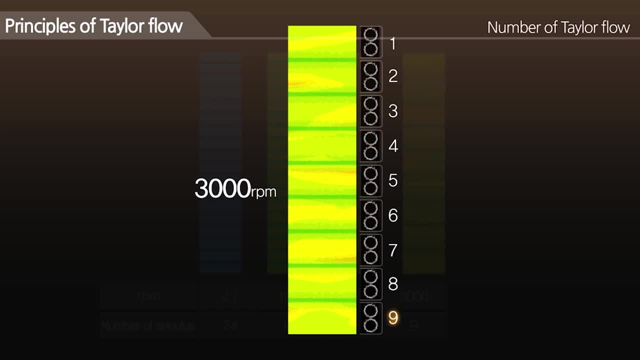 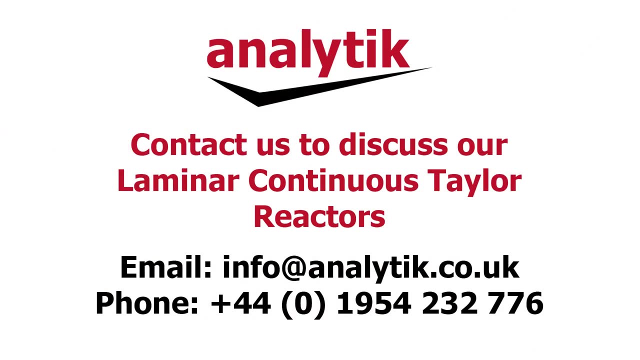 and allow a scalable process by offering low volume laboratory benchtop reactors to production scale machines. To find out more about Laminar continuous Taylor flow reactors, get in contact with one of our specialists. 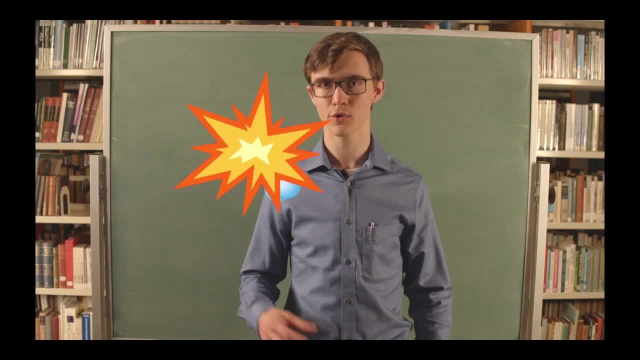 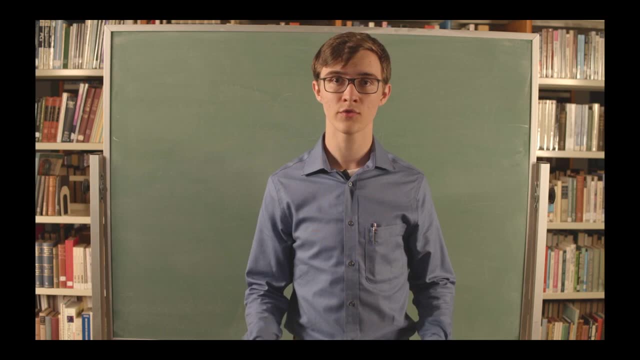 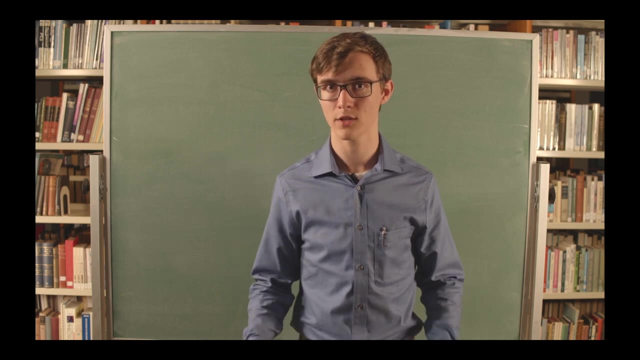 How can nuclear fusion and nuclear fission both produce energy when they're opposite reactions? Well, that's a great question. First, here's a little clue: The fusion of small atoms and the fission of large atoms both increase the stability of the atoms involved. Okay, 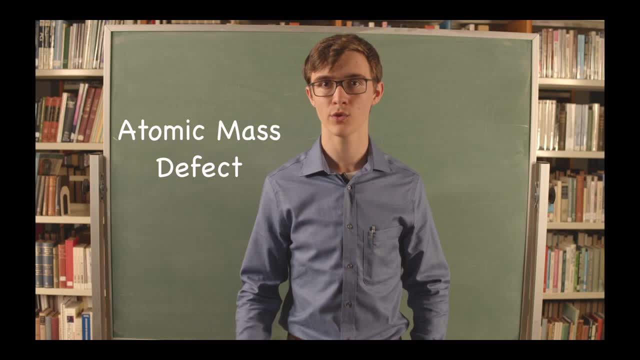 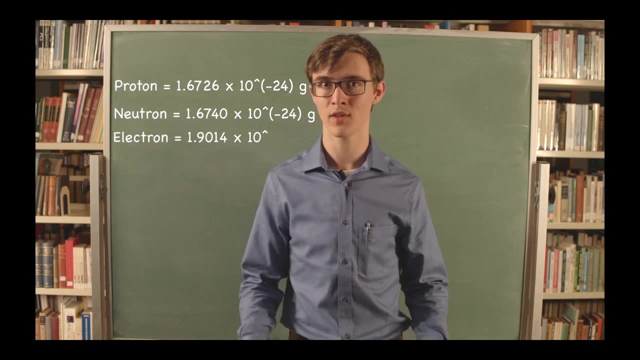 so the key is called the atomic mass defect, which goes like this: Protons, neutrons and electrons each have a specific mass, so when you combine a certain number of them to form an atom, you'd expect the mass of the atom to be the sum of the masses of all the particles in that. 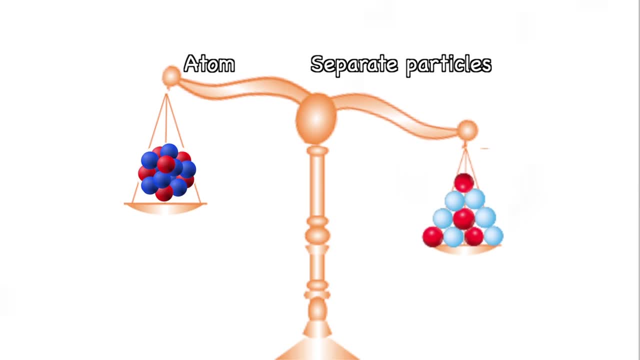 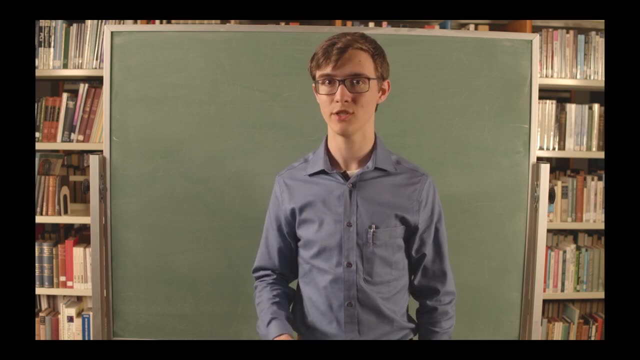 atom, But in fact the atomic mass is slightly less than that sum. This is because the atom is more stable than the individual particles, meaning it requires less energy to exist than those particles. The difference in energy is called nuclear binding energy, and it is the amount of 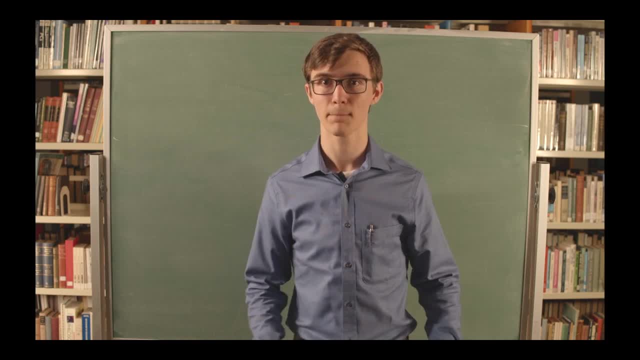 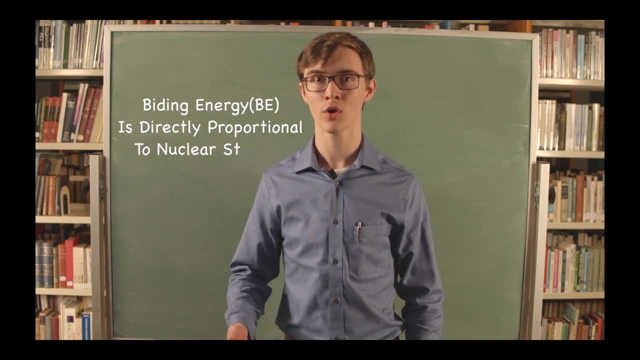 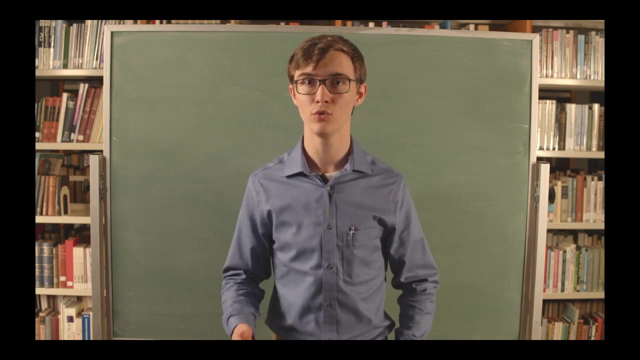 energy necessary to split an atom's nucleus. As atomic mass increases, the binding energy BE also increases, because the atom becomes more and more stable, meaning it requires less and less energy. Therefore, when you fuse two small nuclei, the new, larger nucleus requires less energy than 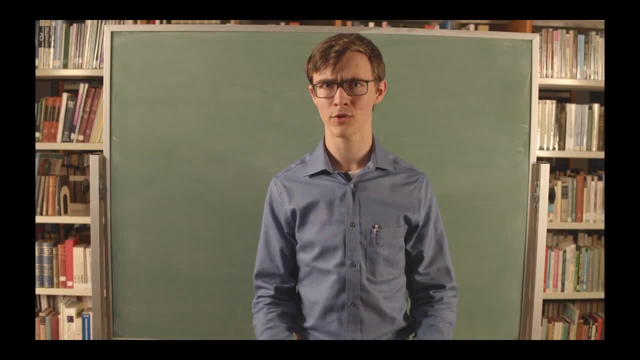 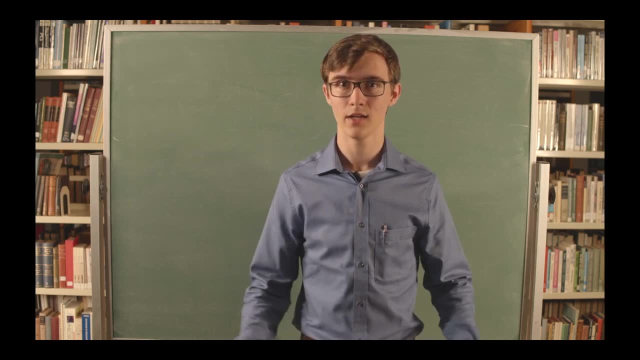 both of the small ones, and the excess is released. Now you might be thinking: if fusion produces energy, shouldn't fission only consume energy? Well, not exactly, See. BE only increases to a certain extent. Iron-56 is the most stable element and 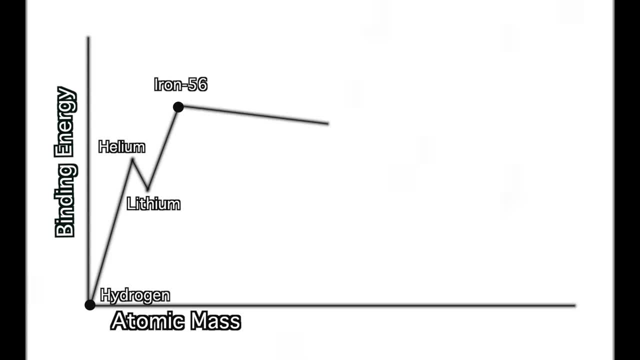 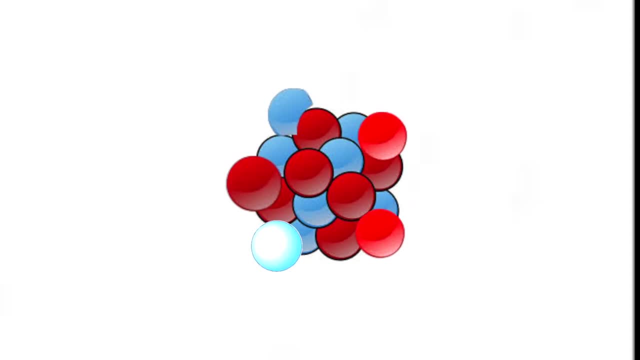 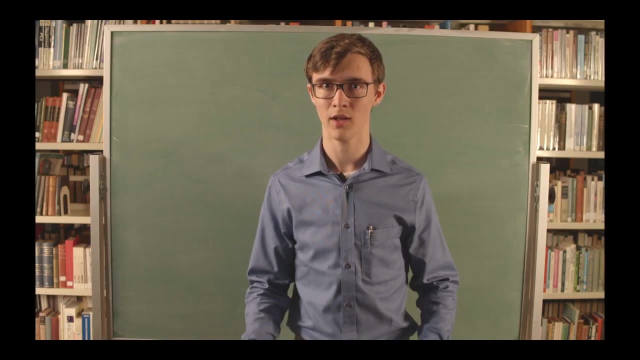 has the maximum BE. Elements larger than iron begin to decrease in BE because the strong force which holds the nucleus together has less of a pull on the particles near the edge of the nucleus, making it unstable. Therefore, when you fission a heavy, unstable element into lighter,